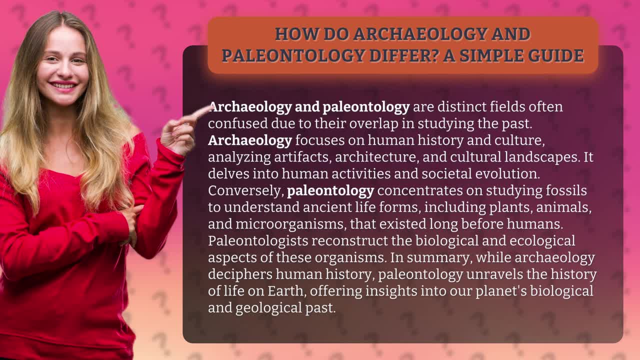 life on Earth, offering insights into our planet's biological and geological past. Thank you for watching. 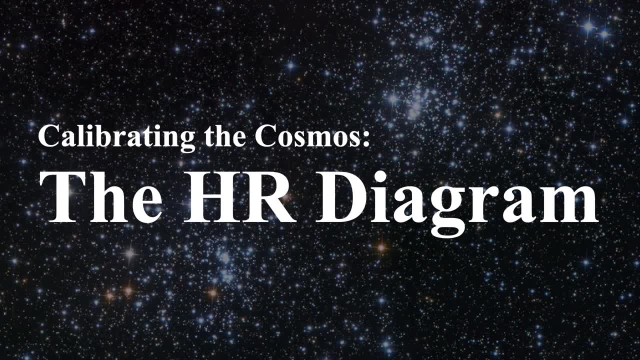 Hello, this is Jason Kendall. Welcome to the next of my introductory astronomy lectures. Now we've gotten to the point where we can actually put a lot of things together, from the spectral type to color diagrams, to distances, to luminosities, to temperatures. 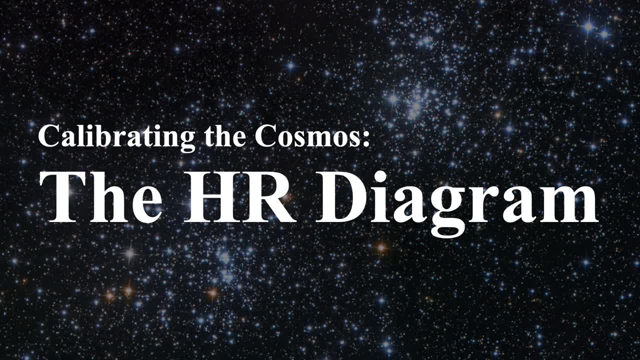 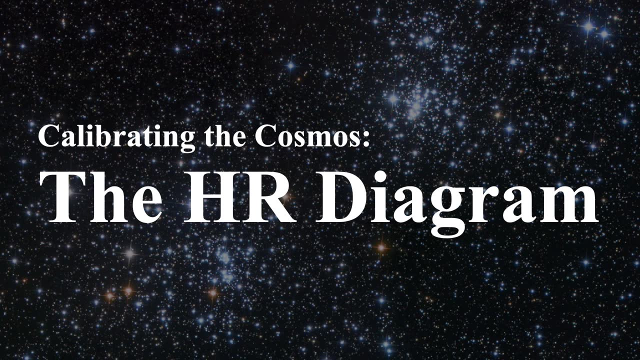 to everything and masses to create one of the most important tools for all of astrophysics that tells us enormous amounts of information about the types of stars, their futures, their histories and their destinies and their origins, And it's called the HR diagram. 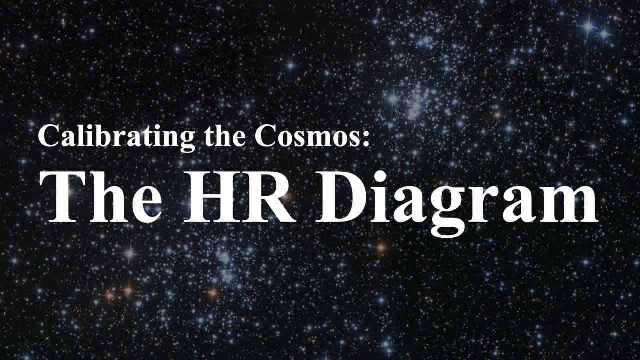 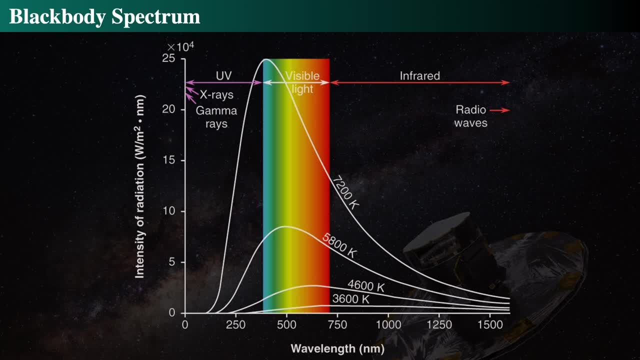 or the Hertzsprung-Russell diagram. So let's see what that is. It's one of the most important tools for all of astronomy. Let's check it out. All right, let's go back and get some of our basics together. All stars are very well approximated by having their spectrum be. 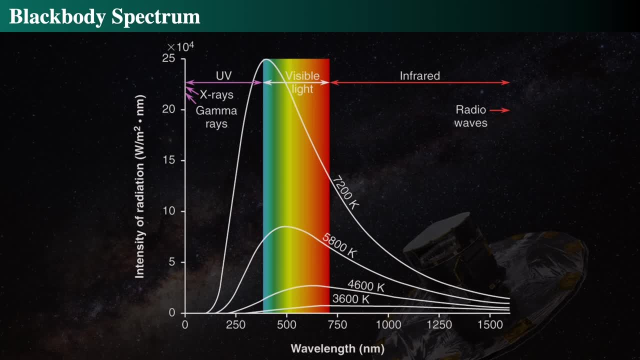 what's called a blackbody spectrum, And a blackbody spectrum assumes that the object is hot and dense and that the light can go inside in it and bounce around until it's completely what we say thermalized, so that all of the material inside of the star is roughly the same. 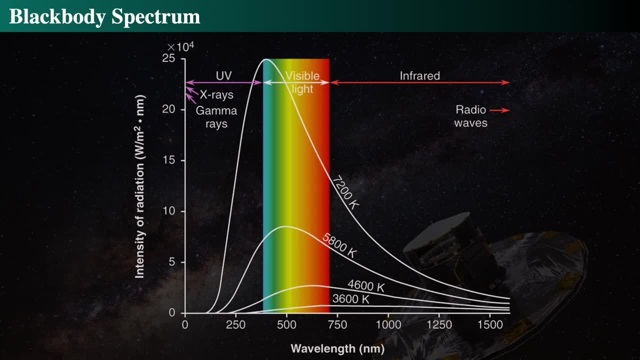 temperature And as it emits from the surface- well, that's kind of dicey for the star, but right at the surface it becomes the same temperature. And as this light emits from the star, the surface across the entire thing and can be described by what's called a blackbody, And a blackbody has.